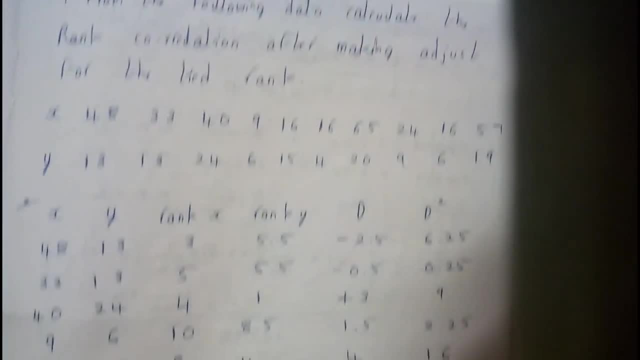 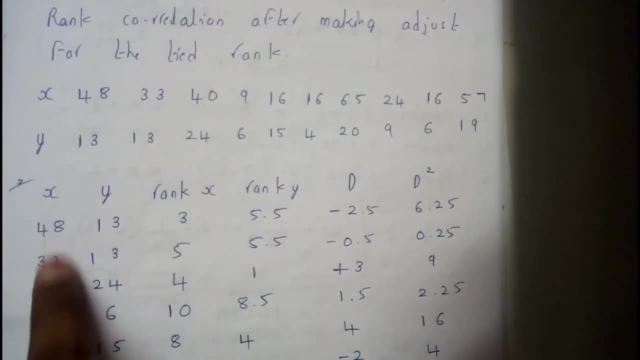 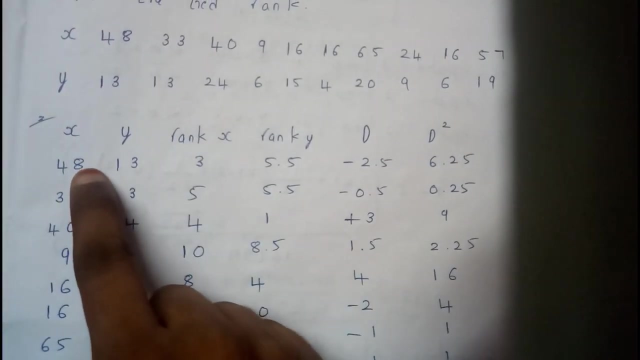 is saying that there are some tied ranks. So basically, x values, y values are given, So x is the. let us assume the marks in one subject, y is in another subject, So we will be assuming the ranks right. So now let us observe here what is the greatest value, guys? 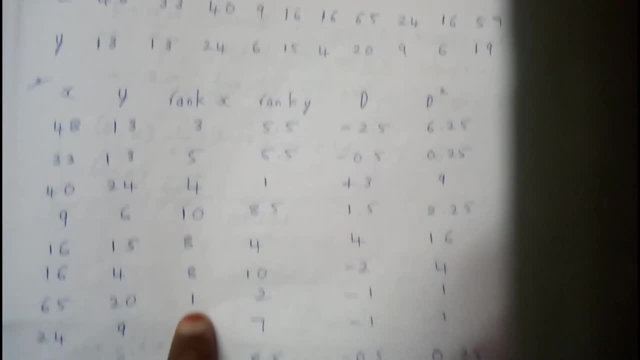 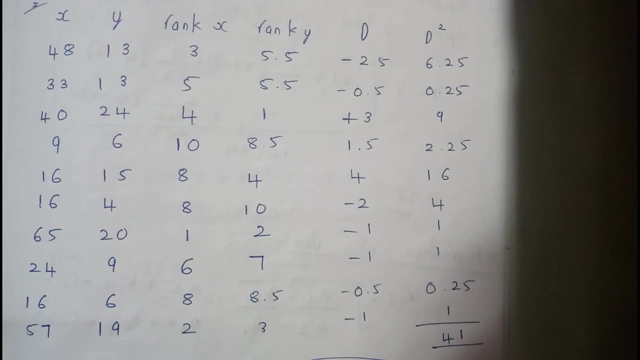 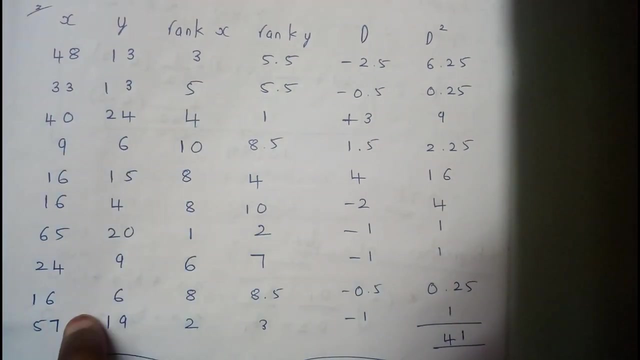 65, right? So at the rate 65 you write 1.. Okay, let me place it properly. Okay, fine, these are all the ranks, Okay, so basically, the 65 is the highest in x, So that will be 1.. The second highest after 65 is 57, right? Yeah, 57 is the second one. Third one: yeah, 48 will. 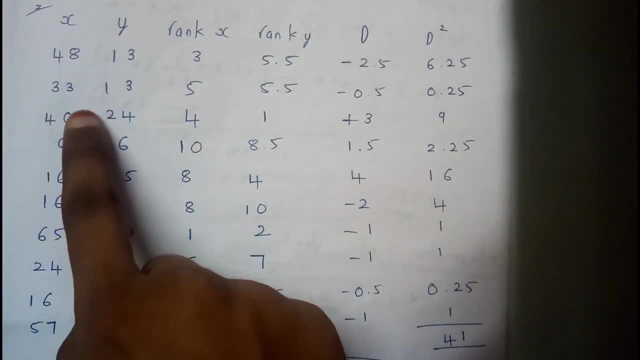 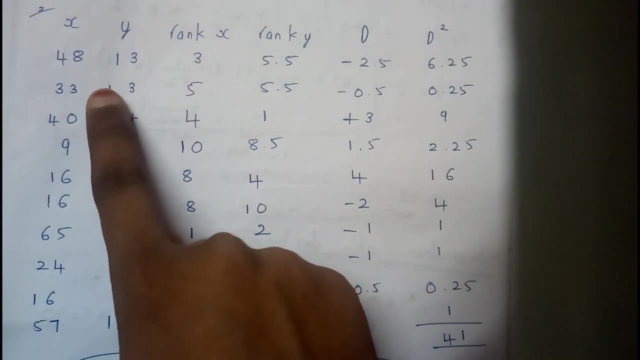 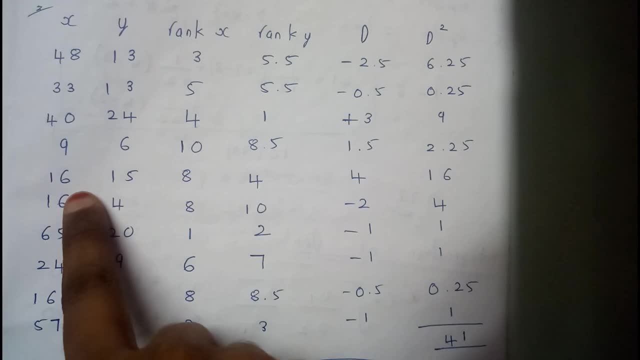 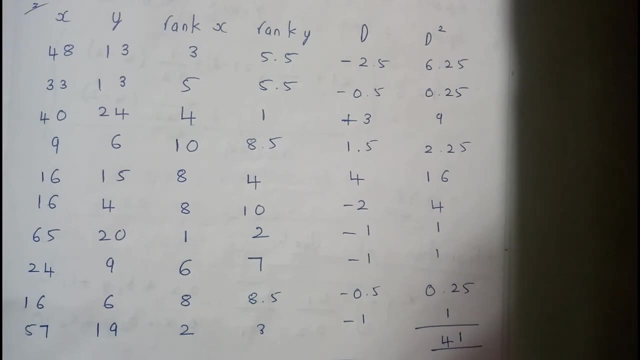 one 24.. Okay, after that 16.. But there are 3 16s, guys. That's the most important thing that you should identify once you see the same numbers again. So 16.. There are 3 16s and we came up to 6.. So the 6th rank is done. So the 7th rank is done. So the 7th rank is. 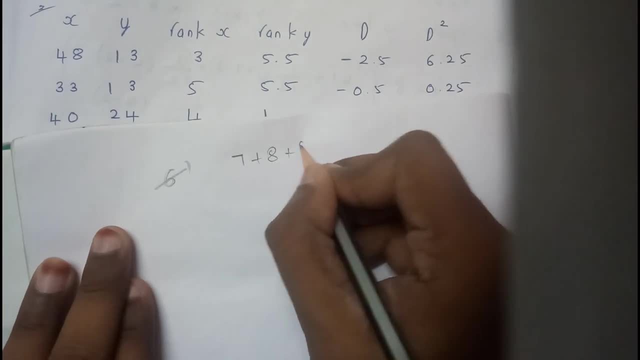 done. So the 7th rank should be 16.. The 8th rank should be 16.. The 9th rank should be 16.. So the total number of ranks is equal to 3. So the value will be 8.. So here, sorry. 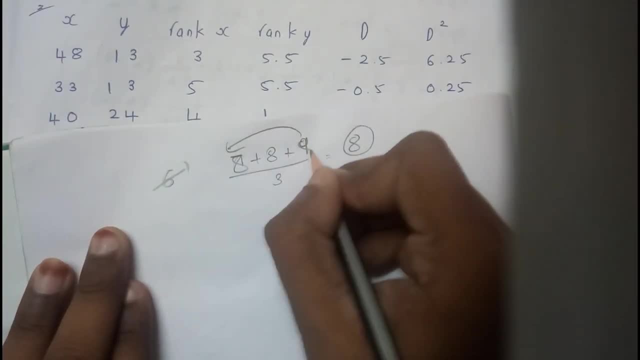 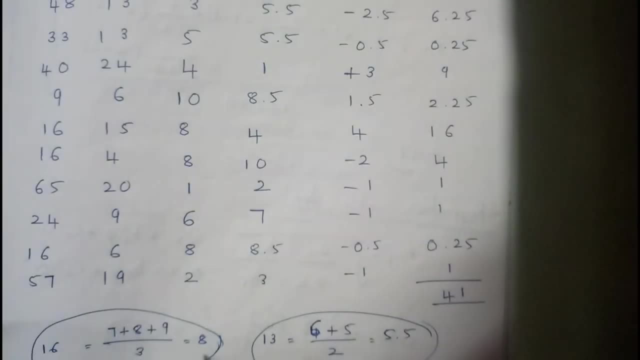 8 or 9.. It will be 8.. So we will be transferring it here. So 8, 8 by 3,, 8.. Okay guys, Okay, fine. So we got the rank 8.. So at the rate, at 16, you write 8.. At 16, you write 8.. At 16: 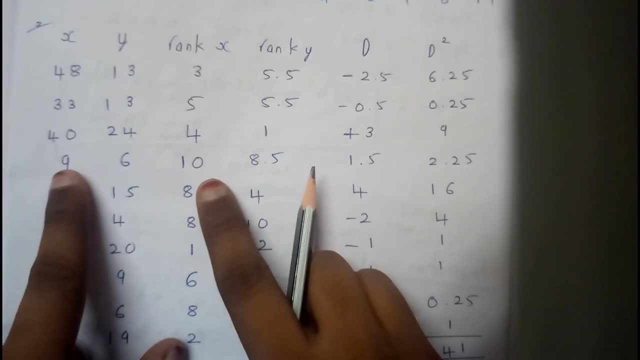 you write 8.. So 9 is already done. So the 10th rank. The 9 marks guy got the 10th rank. In similar way, you will be solving the next two. Why also? So who got the highest guys? 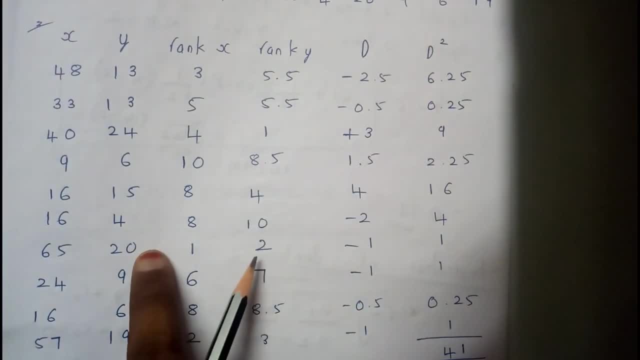 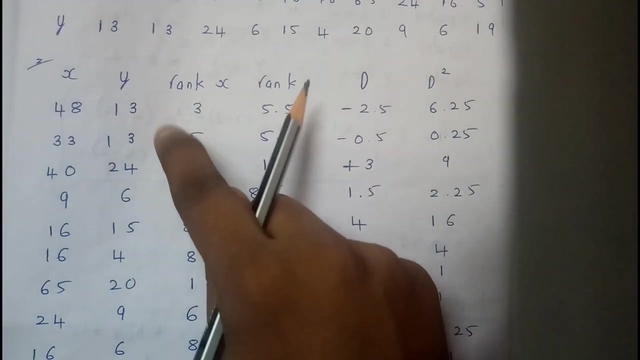 24, right, Yep, 1.. Who got the second highest? It's 20.. Fine, Further moving on, 24,, 20, then 19.. Yeah, 3rd rank. 4th rank could be 15.. Yes, Then the next mark is 13. guys There. 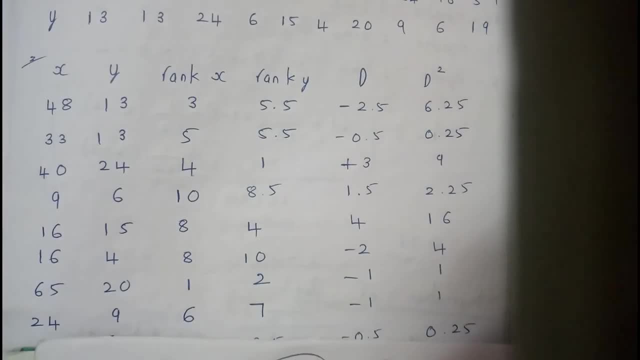 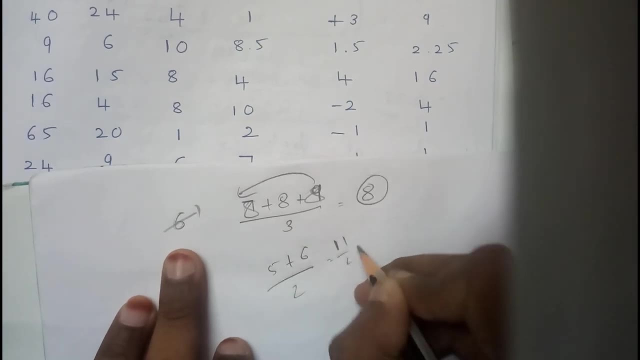 are 2 13s and we followed up to 5th or 4th, Up to 4th guys. So 13 is repeated, 5.. So 5 plus 6 by 2. Which is nothing but 11 by 2. That is 5.5.. So 5.5 will be the ranks. 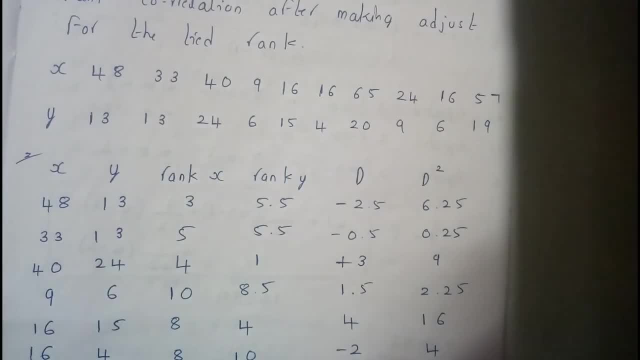 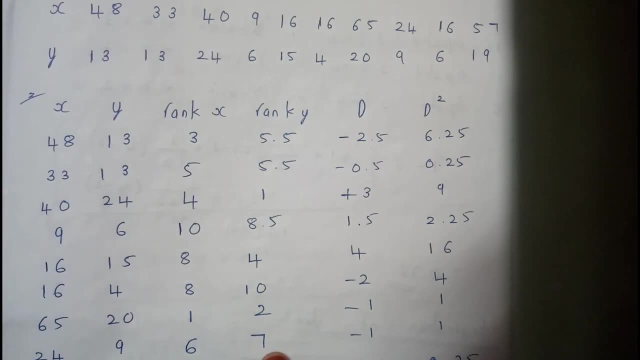 of 13.. So 13, 5.5, 13, 5.5.. Fine, So 6th rank is already done. So 7th rank, Less than 13, what's 9, I think so Yeah, 7th rank And 8th rank. there is 2 possibilities: 6 and 6.. So 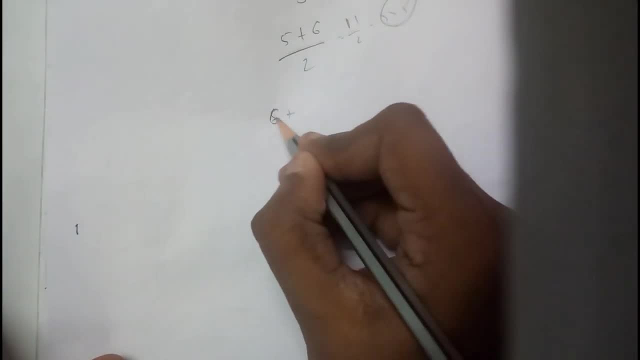 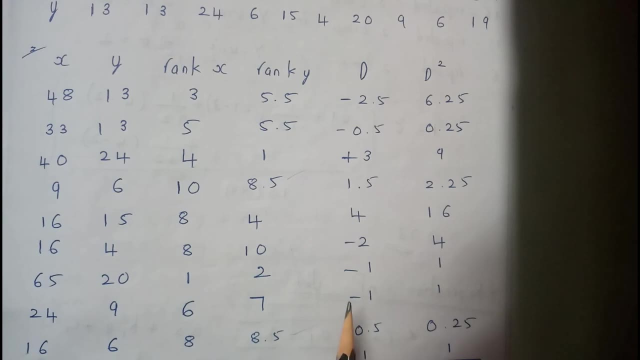 8th and 9th ranks will be occupied by 6.. Sorry, 8th and 9th by 2.. It is nothing but 8.5.. So 8.5, 8.5.. So 9th is also done. So the least guy got the 10th rank, The 8th 8 marks. 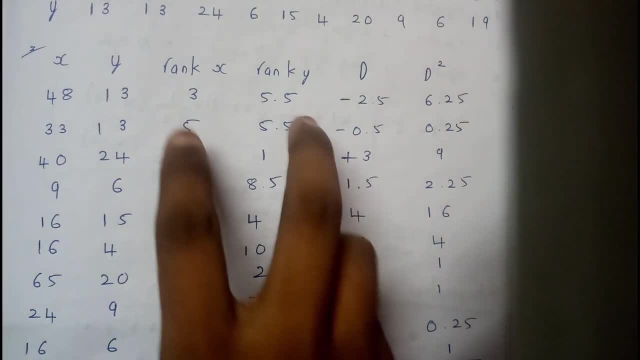 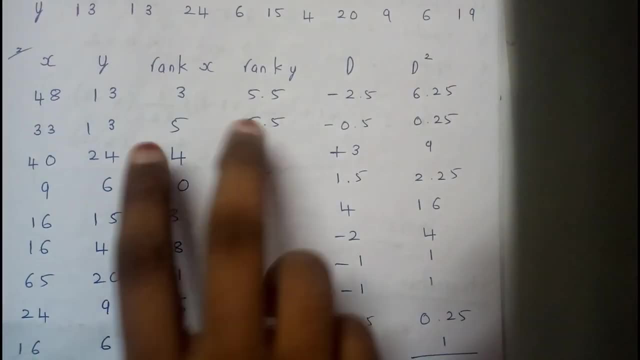 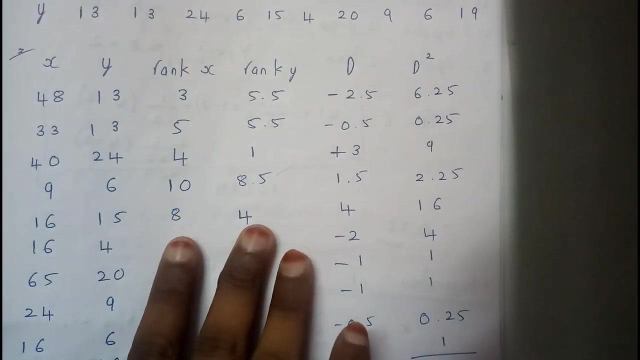 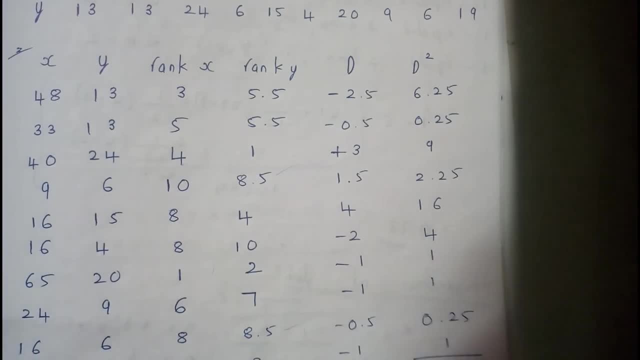 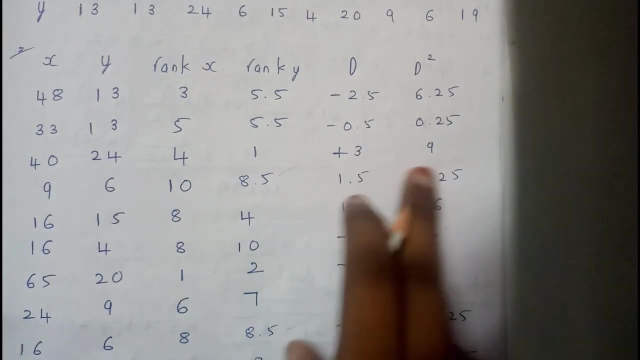 1, sorry, minus 0.5,, minus 1.. Okay, guys, So now I hope everyone got a small idea. So now calculate D squares, which is 25, 625,, 0.5,, 0.25,, 3,, 9,, 1.52,, 0.25,, 4,, 16,, 2,, 4,, 1,, 1,. 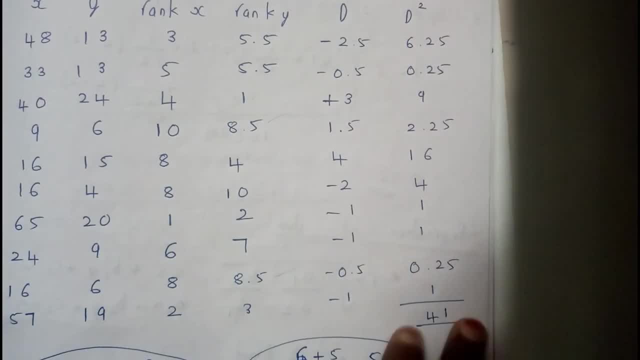 1, 1, 0.25, sorry, 0.5, 0.25, 1, 1.. So we will be calculating D square value. So these are the three things that I have just wrote here, guys. 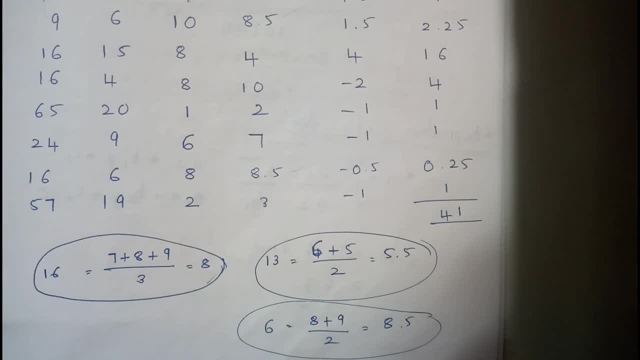 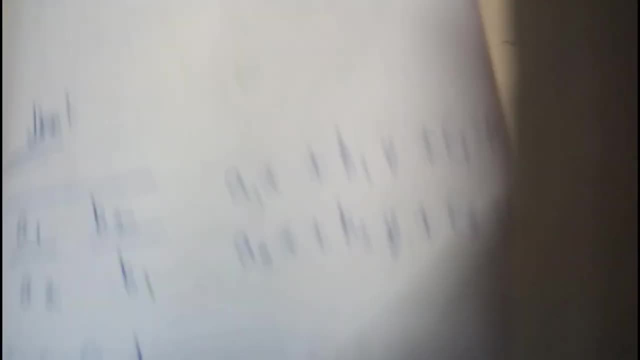 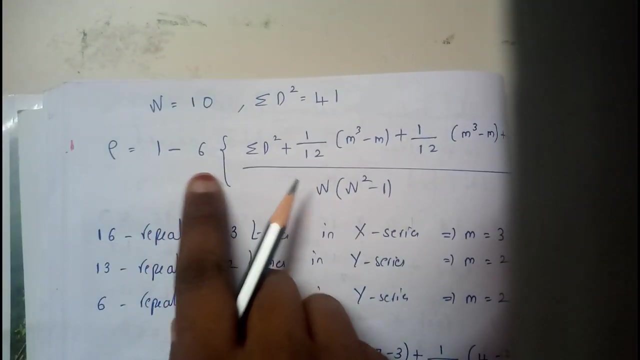 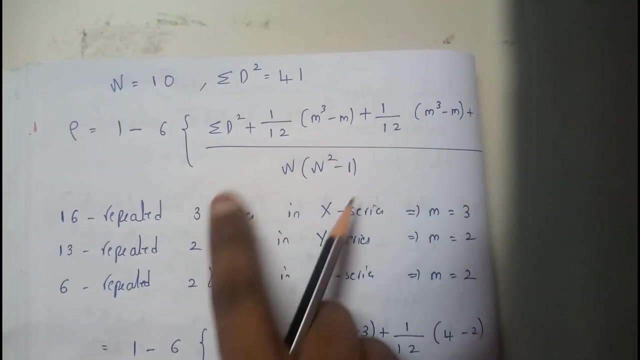 So the things that we have just calculated on the paper with pencil guys. So the value of N is 10 and sigma D square is 41.. Okay, So rho is equals to 1 minus 6 into sigma D square plus 1 by 2 L into M cube minus M, plus 1 by 2 L into M cube minus M, and so on by. 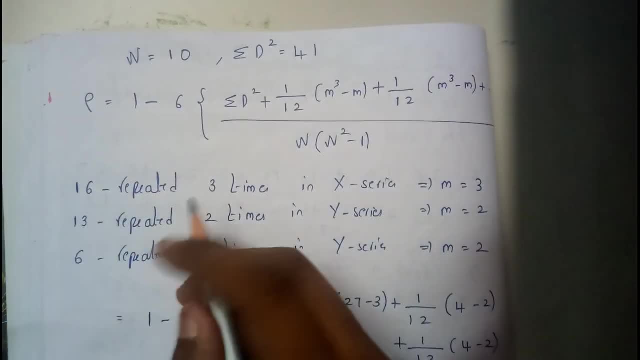 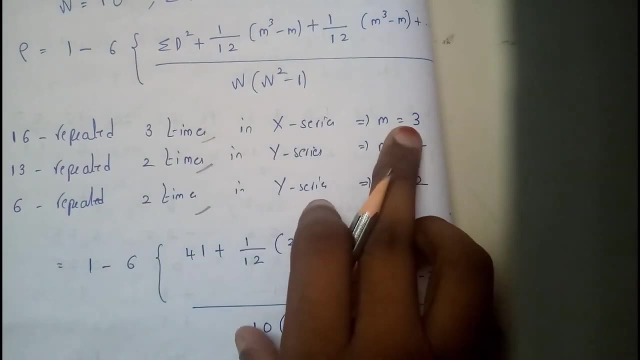 N into N square by N square minus 1.. So 16 is repeated 3 times, 13 is repeated 3 times, 16 is repeated 2 times and 6 is repeated 2 times. So in this case M equal to in this: 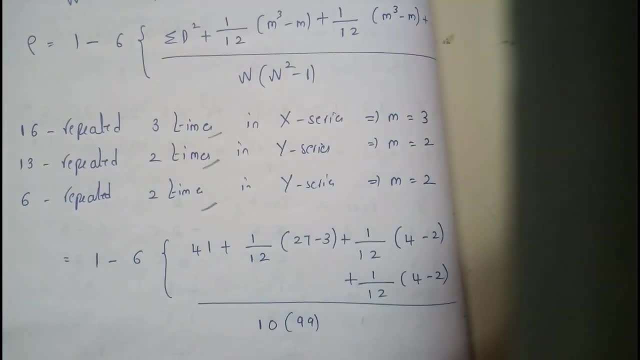 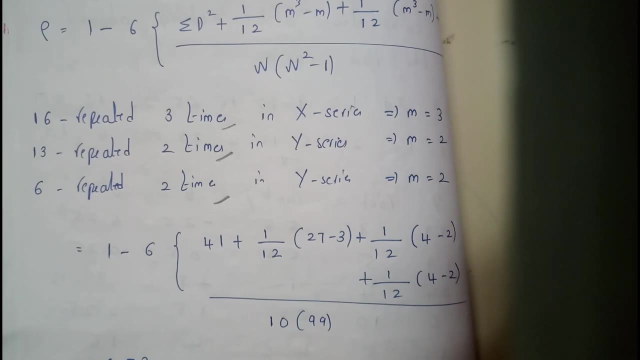 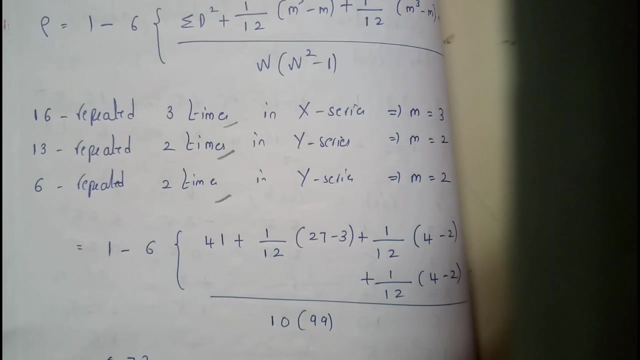 case M equal to 2, sorry, M equal to 3 to 2.. Okay, guys, I hope everyone got a small idea on this thing. So now you will be substituting the values, values in the main equation, guys. So once you substitute all these values, 41 plus 1 by 2 L, into 3, cube is nothing but 27. 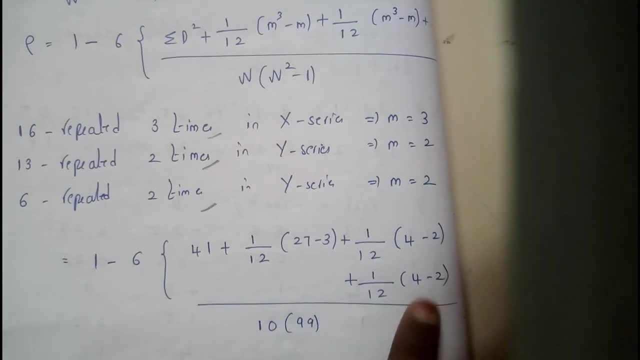 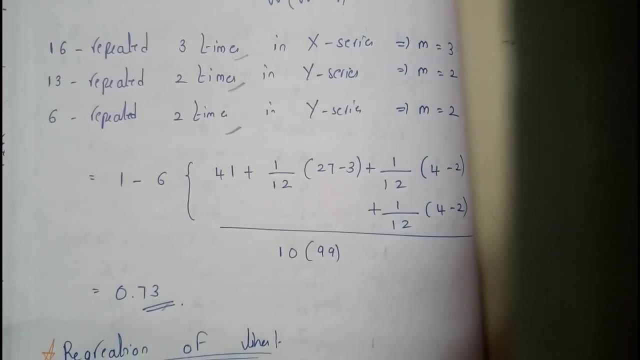 minus 3.. Plus 1 by 2 L into 4 minus 2.. Okay, So I got the value 0.73.. So this is the rank correlation of our repeated ranks, guys. So now I hope everyone got a small idea on the correlation. 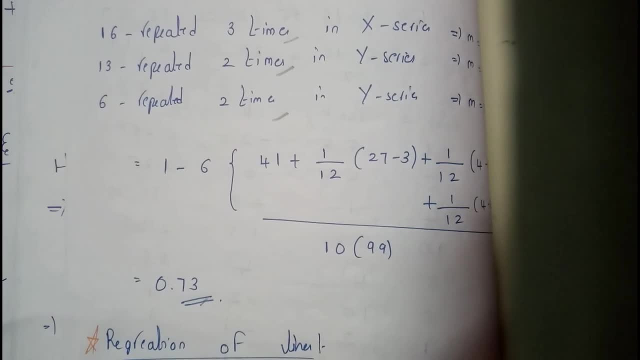 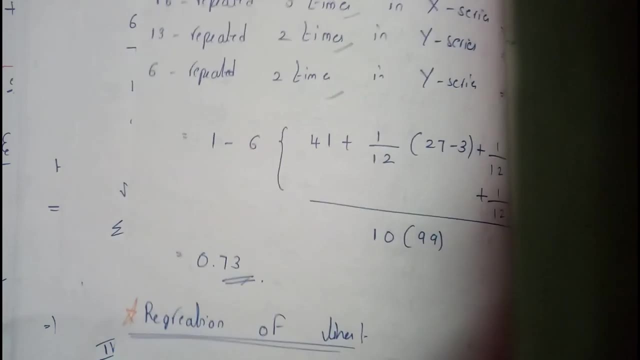 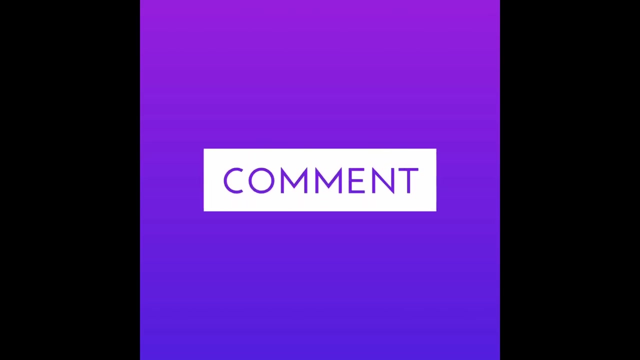 concept. So in the next, in the next videos, we will be going through regression of two lines, guys. Okay, Thank you. Thanks for watching. 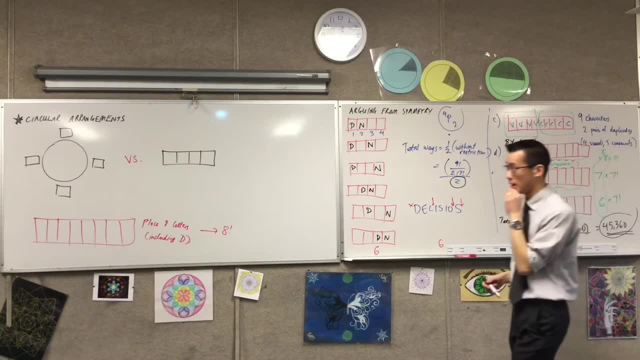 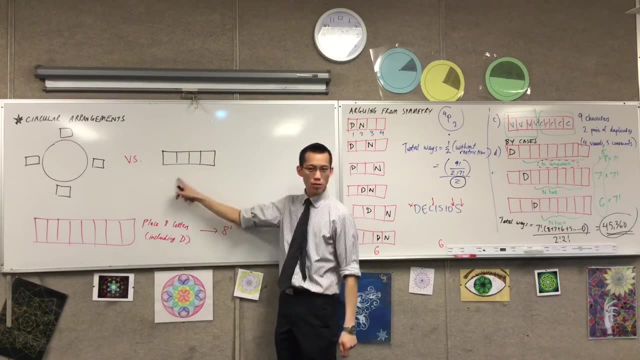 Circular arrangements are a particular subset of questions you'll get in POS and COMs and it's really just one trick to which I want you to understand conceptually. okay, Let's have a look at a normal situation, Just arranging, for instance.